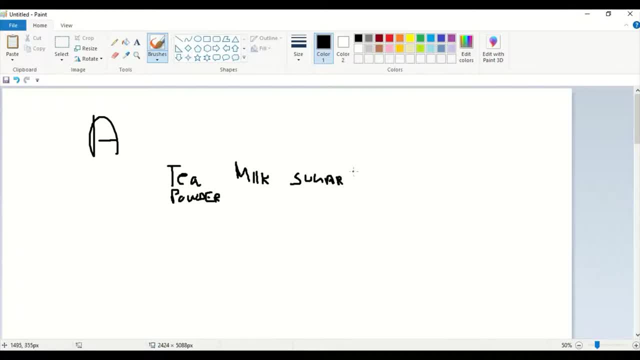 right, if someone is going to take tea powder, he'll go for milk and he'll go for sugar. there is a dependency between these three. okay, this is called a dependencies between each and everything. uh, the dependency between milk and sugar and tea and milk, tea powder and milk, and so on. 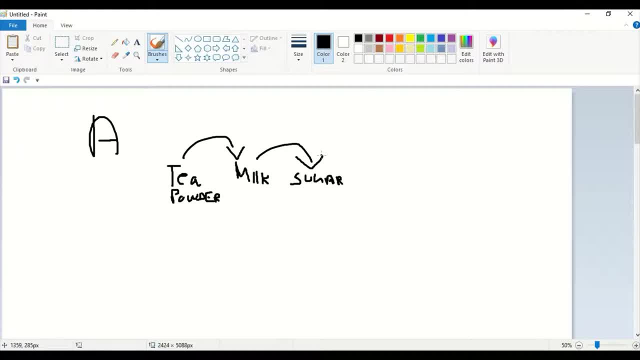 there'll be dependency between each and every product. right the dependency is found out. that is called association. another example for this right: like we can take rice: okay, rice, rice, rice, rice, rice. then if someone is picking rice, he may pick doll as well, doll then as well as salt. so the dependency between the rice and doll has a. 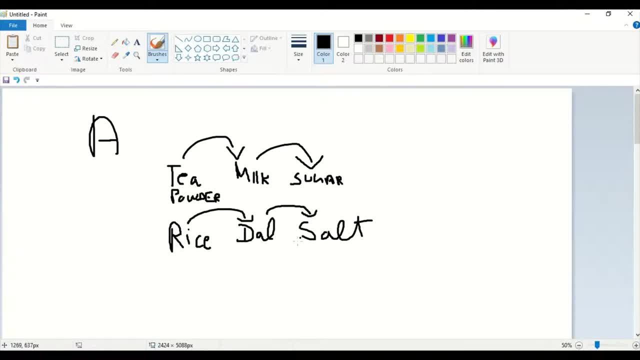 dependency: doll and salt as a dependency. this dependency, how we found out? the dependency between each and each right, each items right. that is called association. there are some set of rules for this association that has. that is called association rules. okay, association rule meaning the set of rules are association rules. 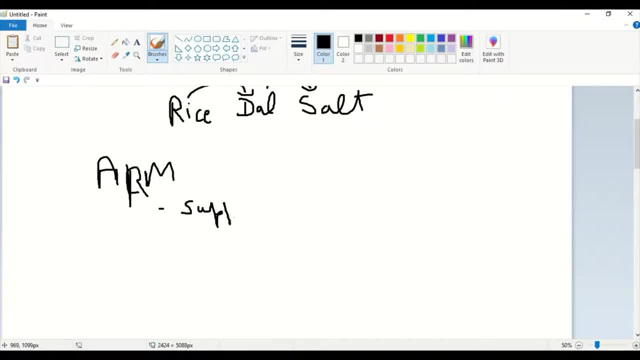 first one is the support. support is one of the rule, one among the rule. then confidence, then last is the lift, then last is the lift, then last is the lift. this is the lift. These three are the set of rules. ok, these three are called rules for association. 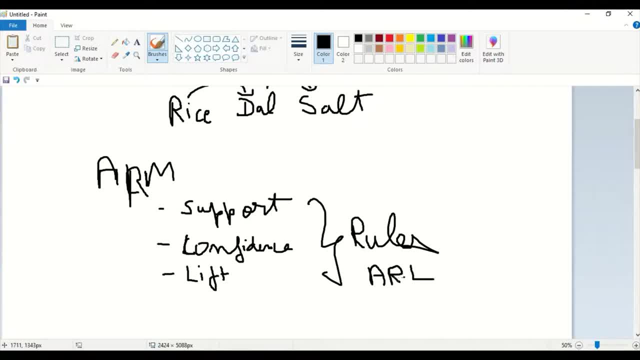 These are the rules for the rules for doing the association thing. ok, Support is the first one. second one is the confidence, third one is the lift. ok, These three. with the help of these three, we will come to know what is the association between two products. ok, 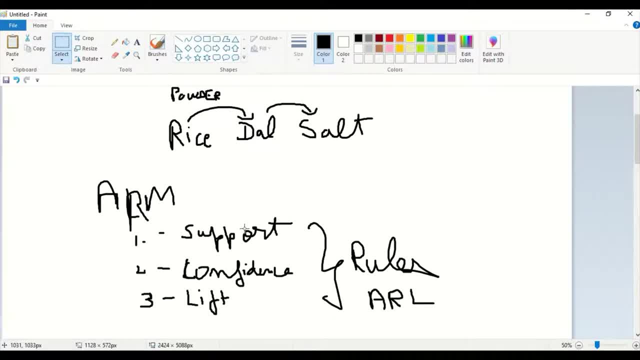 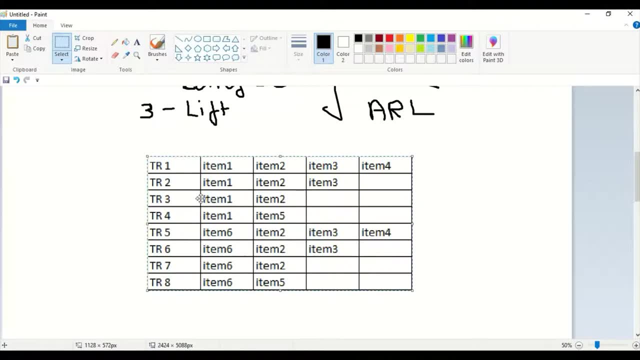 Now how to form this, these three rules, ok. how to find the value for support, confidence lift. ok, We will see the formulas now. This is a small data set right: transaction 1, transaction 2,, 3,, 4,, 5,, 6, transaction. 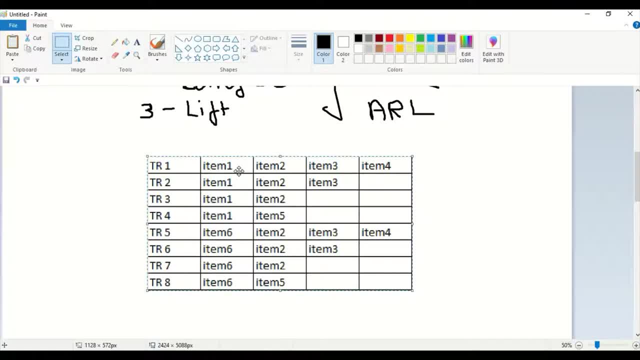 8. ok, there are total 8 transaction. Instead of milk tea powder or rice, we are taking an item 1, item 2, item 3, item 4, like just giving a code name for it. ok, Transaction 1 consists of the item 1, item 2, item 3, item 4.. 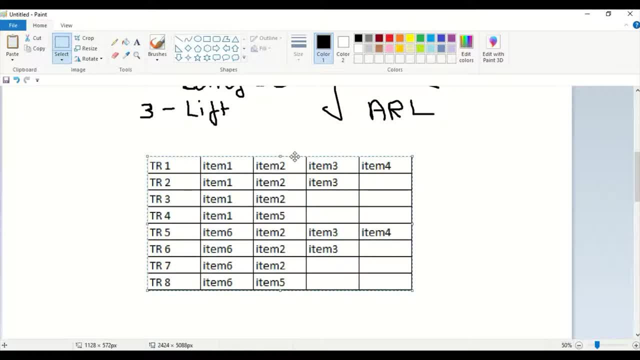 Transaction 1 consists of the item 1, item 2, item 3, item 4.. Transaction 1 consists of the item 1, item 2, item 3, item 4.. The person has taken item 2,. the same person has taken item 3 and item 4 as well. ok, 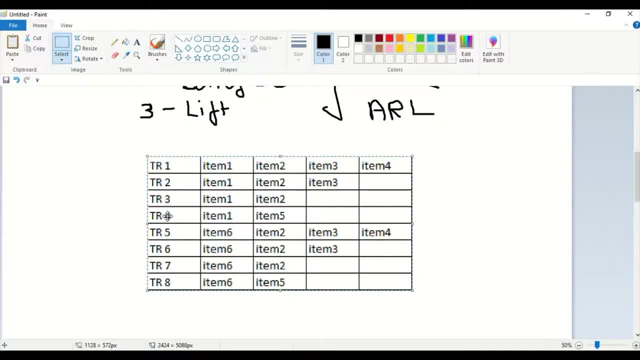 The transaction 4, transaction 4 right: a person has taken item 1 and item 5.. He has not taken item 3,, 2 or 4.. In the transaction 5 right, item 1 he has not picked up. he has taken 2,, 3,, 4 and 6. 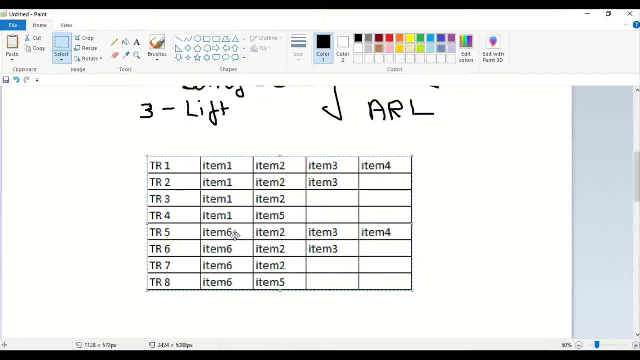 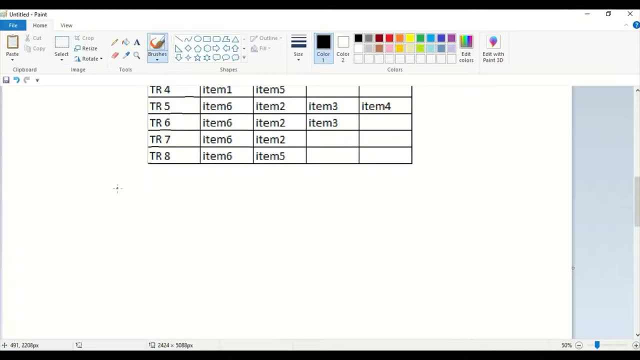 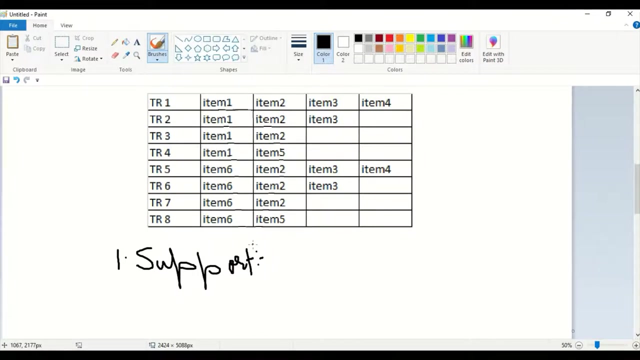 in the transaction. 5. Depends upon the person to person what is coming to take a buy from the store. First of all, we will find the support of this ok. First one is a support. First one is a support. Support is that in item 1 right? 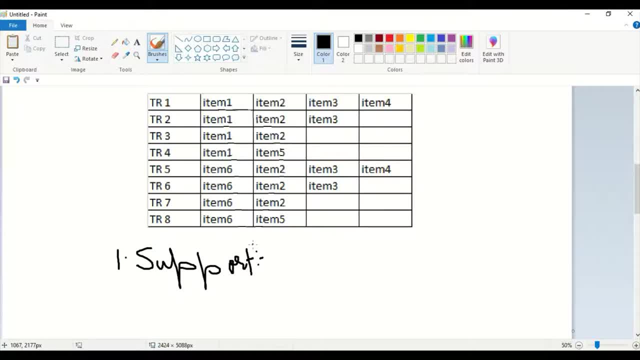 How many transaction has been happened for that item 1 alone? ok, Support equal to in the total number of transaction. item 1 has been appeared for 4 day, 4 times that is 4. transaction item 1, 4 times that is 4.. 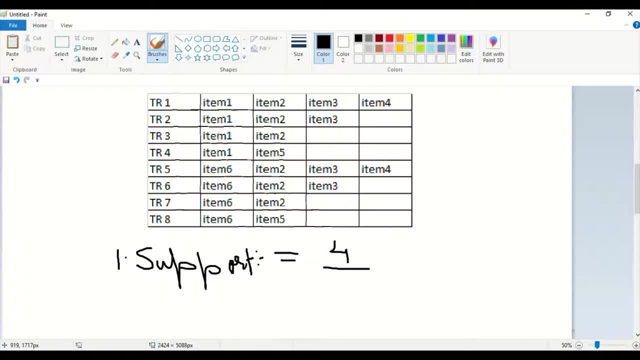 But the total transaction for that day is: the total transaction is right, it is 8, it is 4 by 8.. This is support for item 1,, 4 by 2 as a support which is equal to some value for others. it. 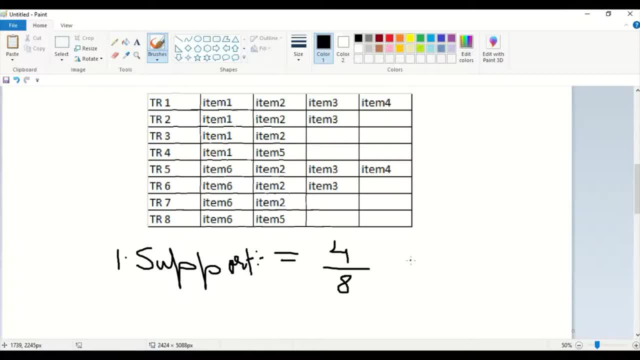 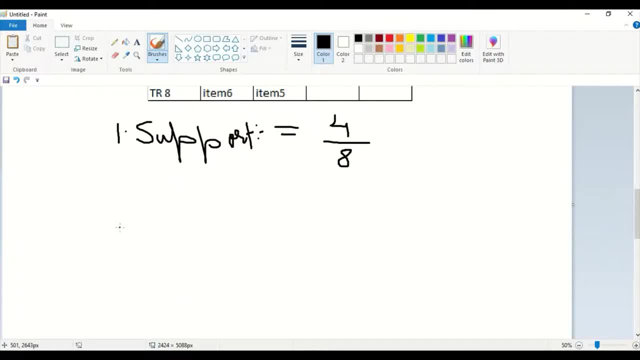 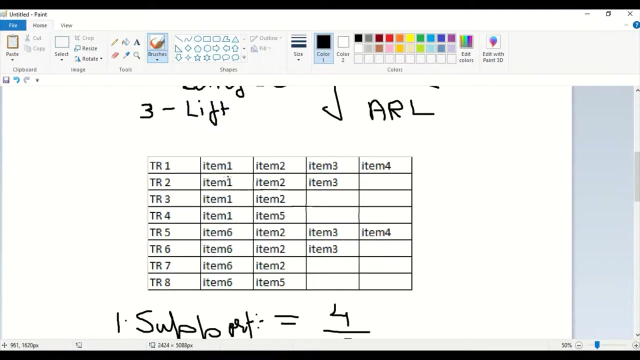 will be like 1 by 2, this is simple data set. For complex data set, we will find out how it is ok. Next one is right. Second one is the confidence Confidence support of item 1.. Item 1 is: 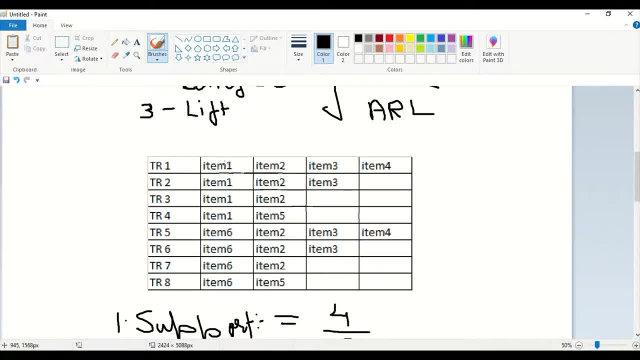 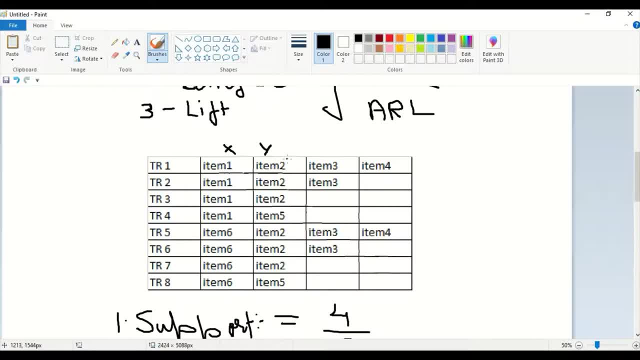 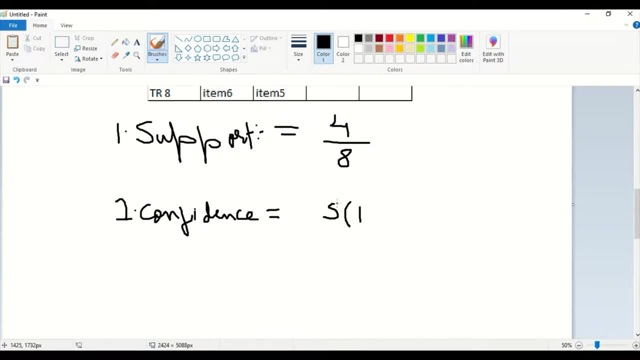 the item y is bought ok, Whenever y comes. what time, like, x is getting bought ok, which is coinciding association between both item 1 and item 2.. Support of 1 and 2 by the ratio: Support of 1 because we, at what time, like if item 1 is coming, coinciding with the item. 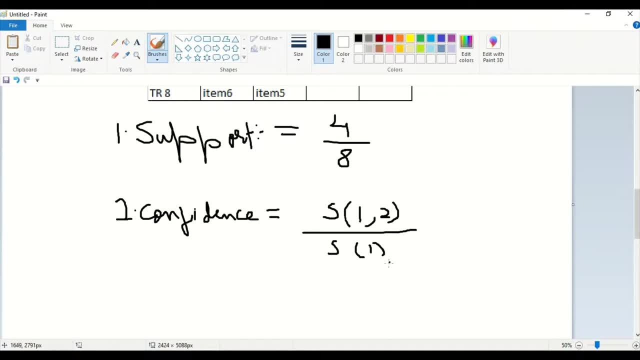 2: ok, This is item 1.. This is for item 2, ok. Confidence of item 1 with item 2.. In correlating the item 1 confidence with 2.. Whenever x or item 1 is bought, how much times item 2 or y is bought along with it? 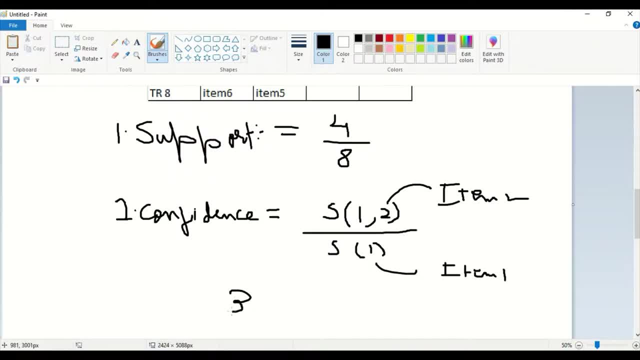 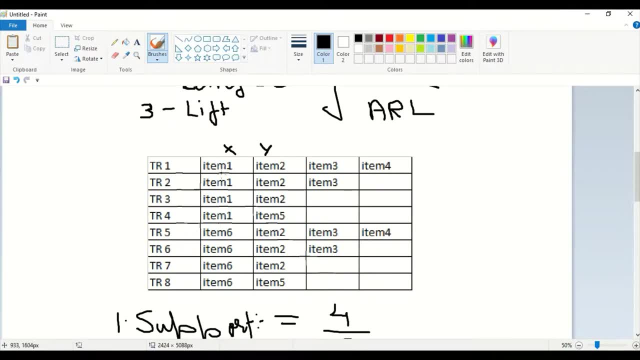 The value right. it will be around 3 out of out of 4.. There are 4 transaction. Item 1 is there In that 4 transaction. 3 transaction are correlating item 1 and item 2. ok, Y value is occurred in 3 times though. 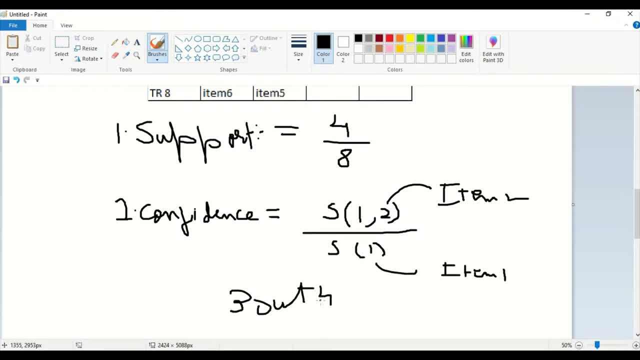 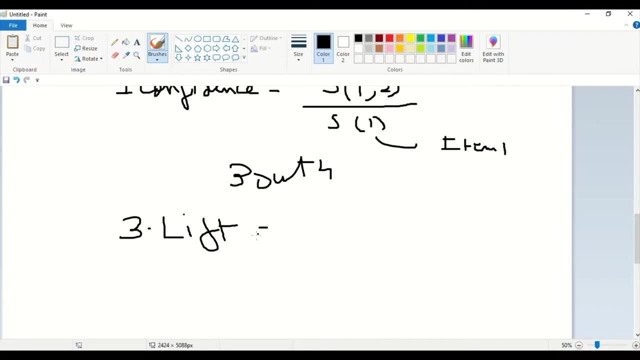 3 out of 4 transaction. that is the confidence of y according to the x. that is confidence of item 2 according to or correlating with item 1. next one is the lift lift. lift is calculated by support of 1 comma 2. 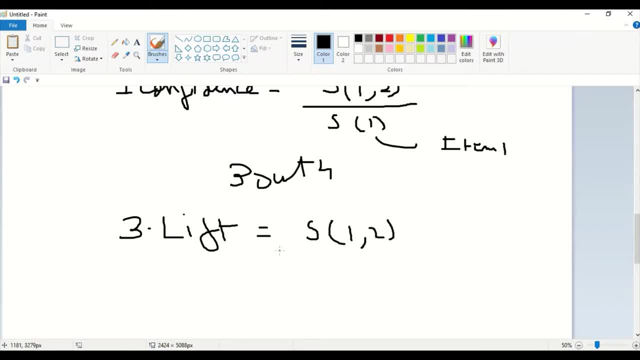 item 1 and 2. support of item 1 and 2. support of 1 into support of 2. that is, support of item 1 into support of item 2. this is gives the like probability of item y. how much time is it bought? 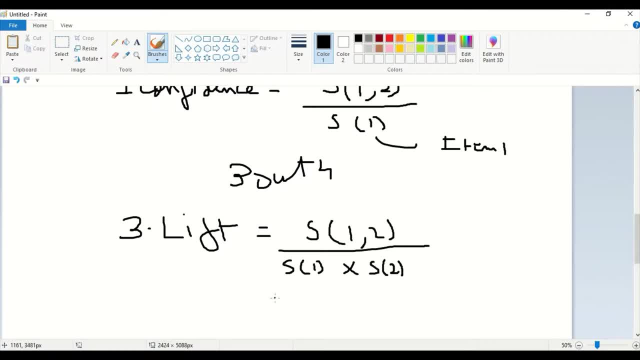 again: item 2 when it is sold. item 2 when it is sold. item 2 when it is sold. when x is bought. okay, that is, item 1 is bought. i am taking milk at how much times, or like milk or tea powder is bought along with milk.